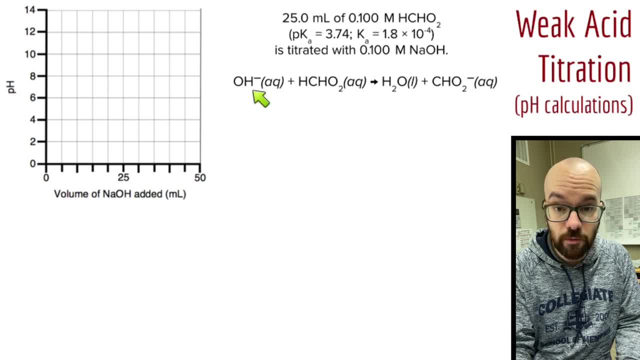 reaction. right here as well, I've got hydroxide ions, that's from the strong base plus the formic acid molecule And that's written together as HCHO2, remember, because it's a weak acid. So it's mostly like this: until it gets titrated And that's going to produce water as well as formate. 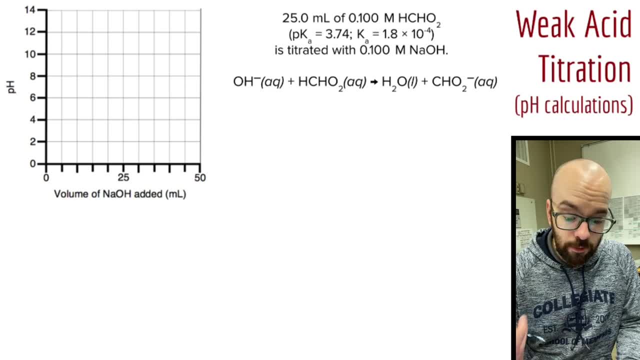 the conjugate base of formic acid. So the first thing that we don't know yet is: how much NOH do we add to get to that equivalence point? So let's just do our quick calculation of that. We'll use, of course, MAVA equals MBVB. Solve that for volume of base in this case, because that's what we don't. 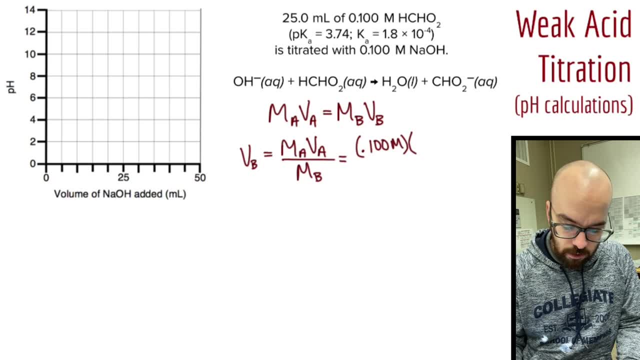 know, And 0.1 molar of the acid, We've got the volume of acid of 25 milliliters And of course we're going to divide by the 0.1 molar sodium hydroxide concentration and we're going to get 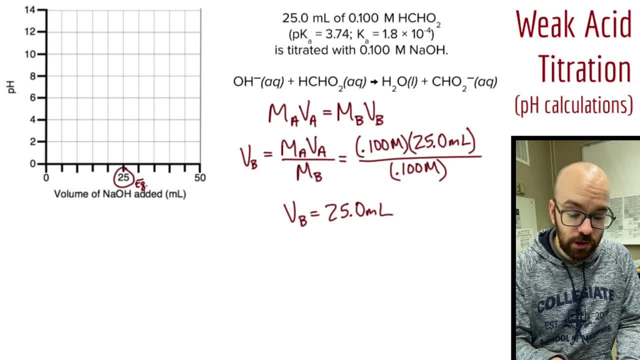 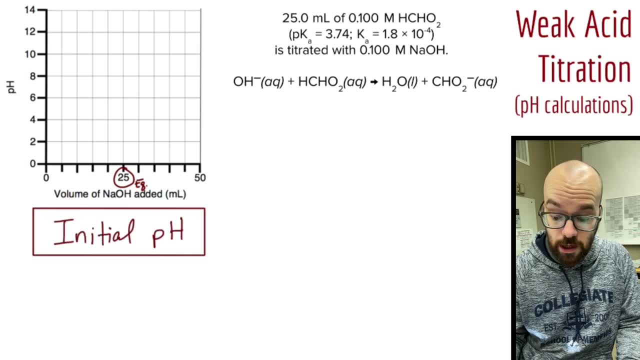 25.0 milliliters. We'll mark that spot on our titration curve right here as our equilibrium volume. And now we're ready to calculate some pHs along this. The first one we'll start with is just the initial pH. So to start off with this, we're going to write the acid dissociation of: 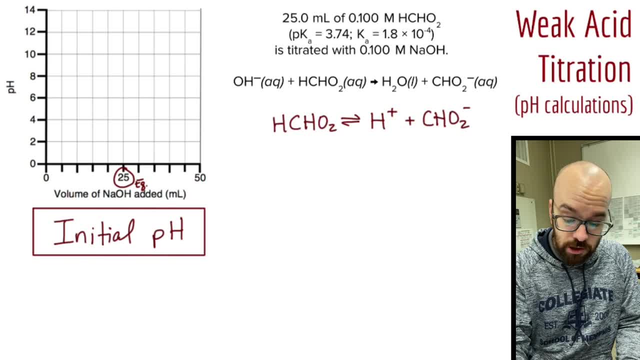 formic acid. So I've got that written here. It's different than the neutralization reaction, of course. The neutralization is like the base plus the acid and it gives us water and the salt. But in this case we're just looking at the dissociation of formic acid, because we haven't 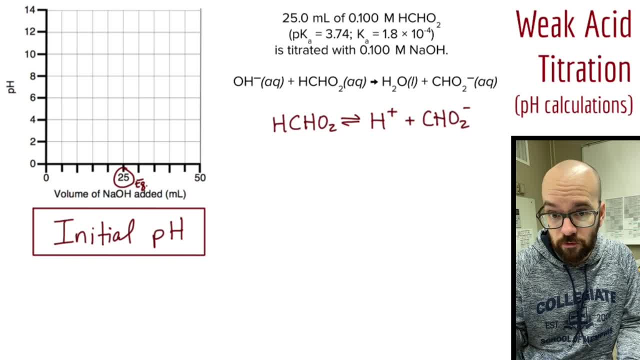 added any base yet. So this is just the normal equilibrium of this weak acid in solution. So we'll start off with an ice table and we've got 0.1 molar of the formic acid and we've got 0. 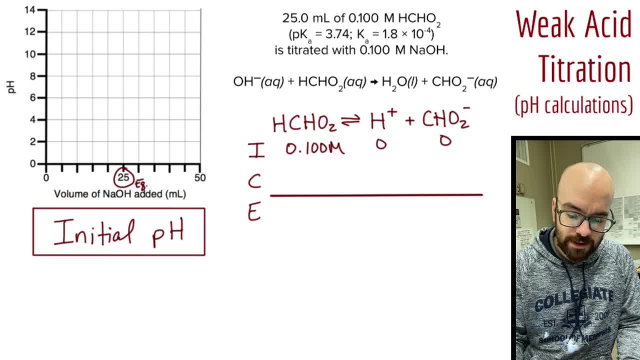 molar of the H plus and the conjugate base And of course that acid is going to decrease by X. We don't know that X yet- And then the other two will increase by X. just a standard Ice table for a weak acid And we get 0.1 minus X and X and X. Then we'll write the Ka expression. 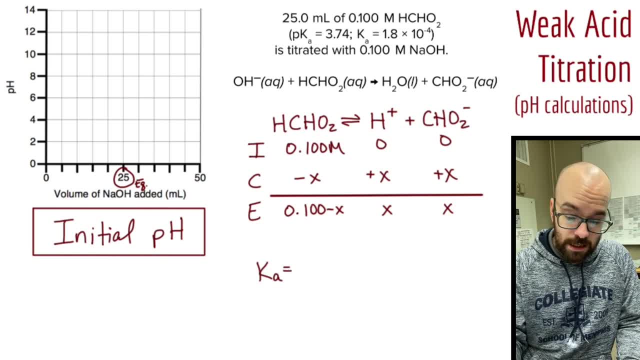 for this, since this is an acid dissociation. So Ka equals, of course, the H plus concentration times the conjugate base divided by the acid, And we'll go ahead and sub in those numbers there. So X times X is X squared over 0.1 minus X. We'll use the X's small approximation that we usually 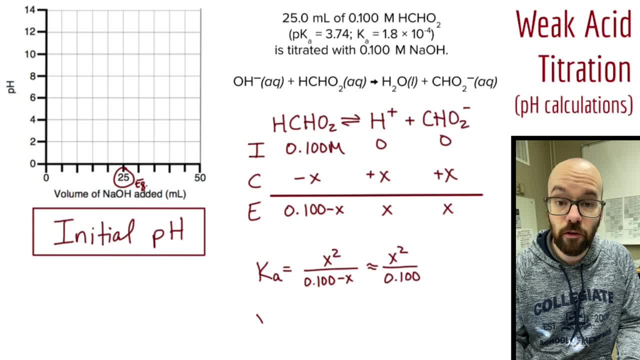 use in these and get X squared over 0.1. And we'll solve for X. X equals the square root of 0.1 times our Ka, which is 1.8 times 10 to the negative fourth And that comes out to be 0.0042426. 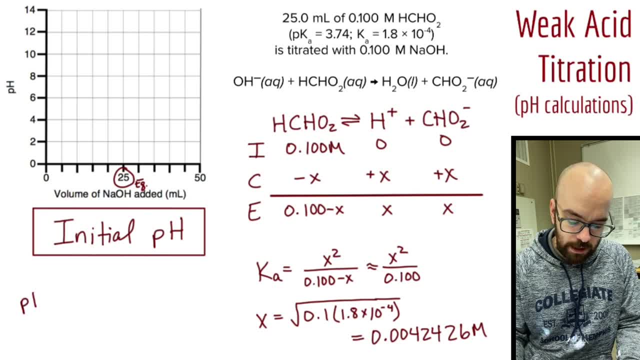 molar, That X is the concentration of our H plus, So we'll take negative log of that to find the pH and we get a pH of 2.37.. I went through that really quickly with the assumption that anybody watching this video on pH titrations of a weak acid strong base titration curve is pretty good. 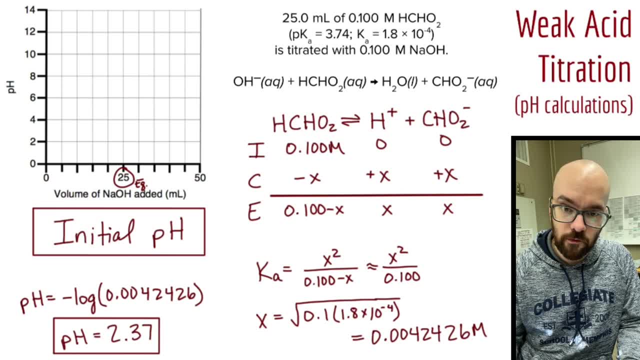 with creating an ice table using a Ka expression solving for pH. But if you need to pause the video so you can work back through, Well, we just went through there. All right, I'm going to plot that initial pH on my titration curve. 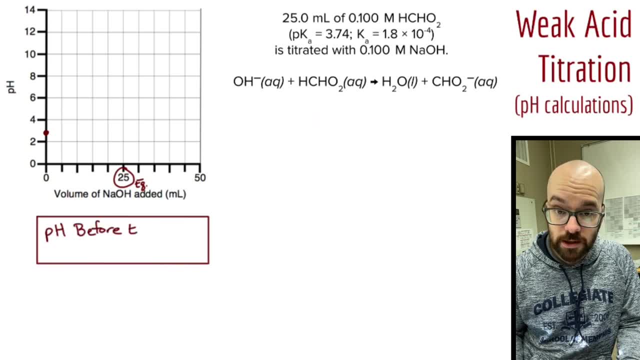 here. I've got that point. All right, now let's add some base. So let's say we've added five milliliters of base, We're before the equivalence point, which is 25 milliliters, remember. So we're. 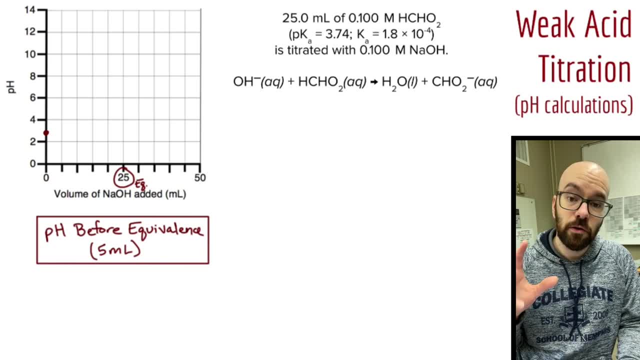 before that equivalence point. And anytime we do this, we first have to do a stoichiometry calculation and then we'll calculate the pH. I always do that stoichiometry calculation in the form of a before-add-after table. Remember, when we do the before-add-after table we have to be 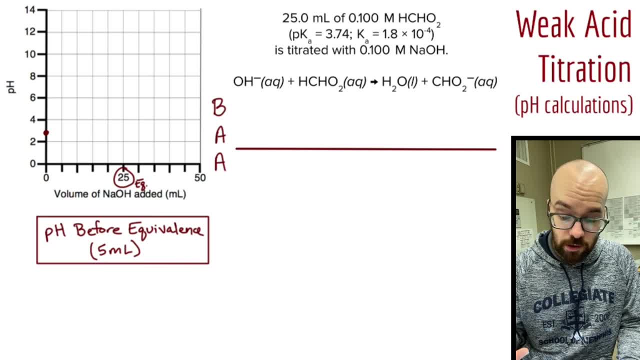 working in moles, because this is a stoichiometry calculation that we're doing: Hydroxide, we have approximately zero, And our acid, let's see, we've got 25 milliliters, So that's 0.025 liters times 0.1 molar and we're going to get 0.00250 moles of. 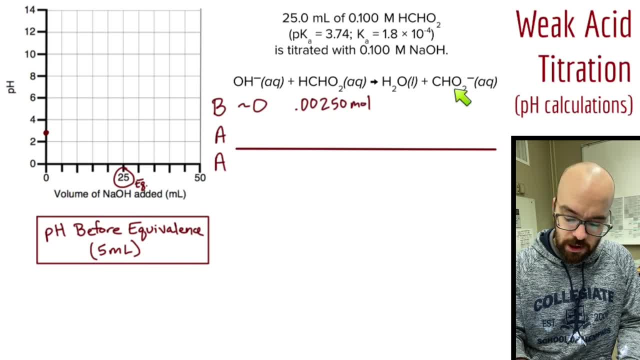 the acid. Also, in our before the conjugate base concentration, we've got approximately zero. We haven't neutralized any of this acid, So technically we'd have a little bit of this, but it's going to be a really, really small amount. So approximately zero. Now let's go ahead and add. 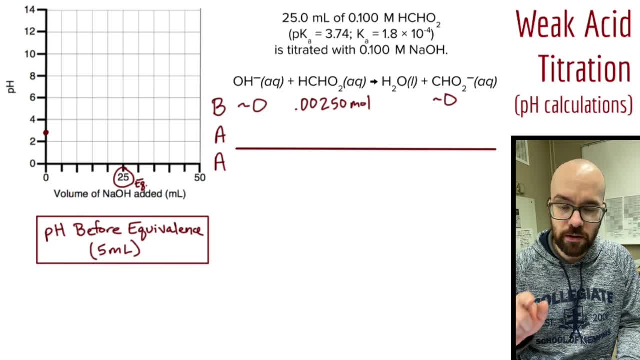 some base. So how much base we're adding? we added five milliliters, That's 0.005 liters. Multiply that by 0.1 molar and then we get 0.0005 moles- Those moles of base. 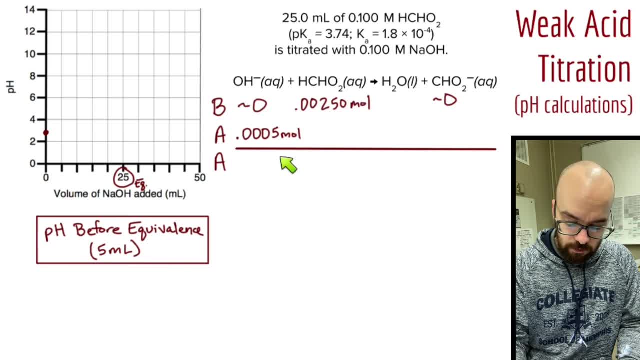 are going to get neutralized by the acid that's already present there, So we'll be left without any hydroxide and we'll have 0.0020 moles of the formic acid left, Of course. what happened to that? 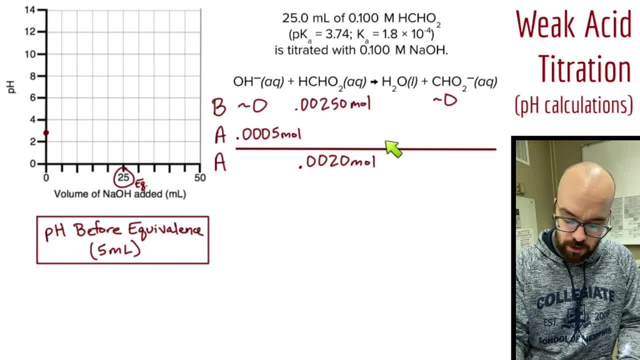 other 0.0005 moles of the formic acid. Well, it was converted into the formate ion or the conjugate base. So we've got 0.0005 moles of that conjugate base. Now here's where we can use a shortcut Henderson-Hasselbalch, because we have a number of 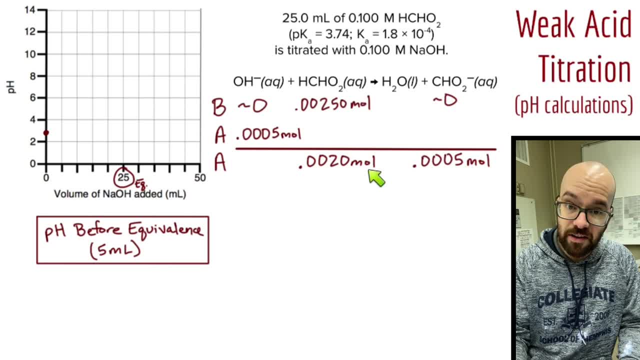 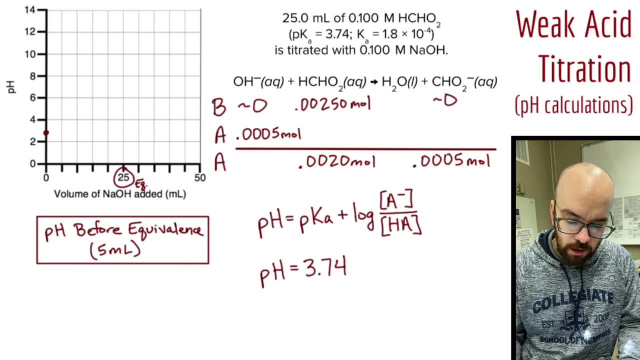 moles of the conjugate base and we have a number of moles of the acid. So we can use those directly in the Henderson-Hasselbalch equation to calculate our pH. That equation of course is: pH equals pKa plus log of the base over the acid. Our pKa, it told us in the problem, was 3.74, plus log of. 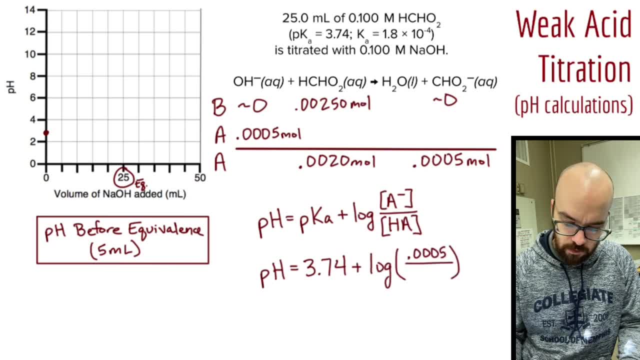 looks like our base is 0.0005, and then our acid is 0.0020.. Now, of course, it's not the same. It's just that we are not using the same concentration. We're just going to keep using the same concentration. So we're going to keep using the same concentration. 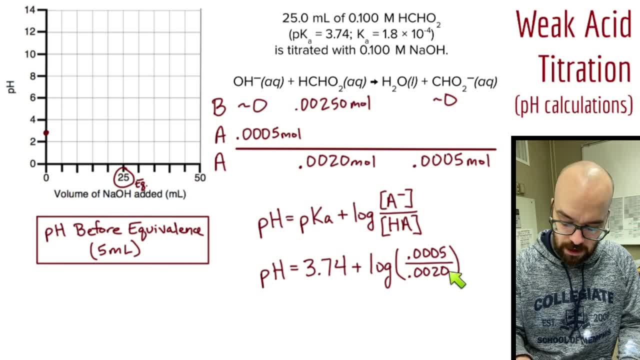 So we're going to do that, And our pH is going to be the same as our concentration. So if we convert these moles into our concentration, we would divide this number by the same volume that we divided this number by. So mathematically that's a wash, It's not going to matter. So we 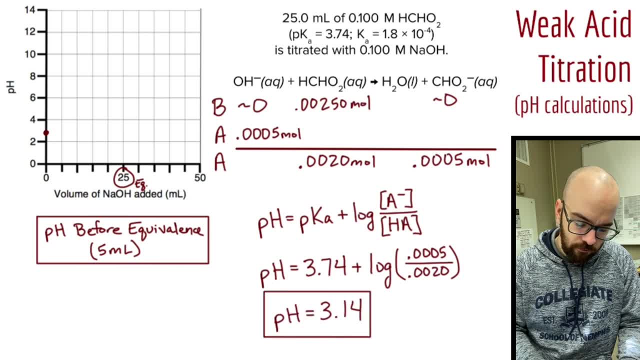 can actually just take the number of moles and go ahead and sub them into this equation, even though it's technically not the concentrations after five milliliters. So I'll add that point on our titration curve right here. To recap that: 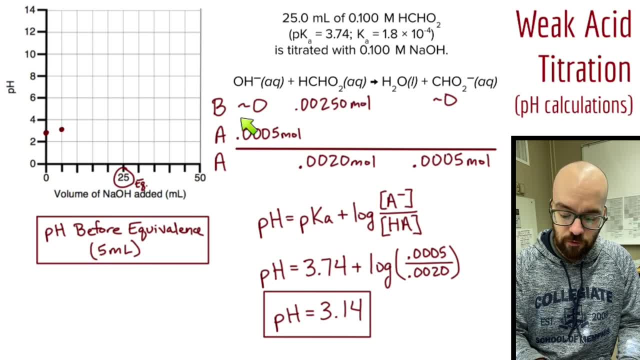 real quick. if we're before the equivalence point but we've added some base, we'll do a before, add after table or a stoichiometry calculation to determine the number of moles of acid left and the number of moles of conjugate base. Then we just use the Henderson-Hasselbalch equation to 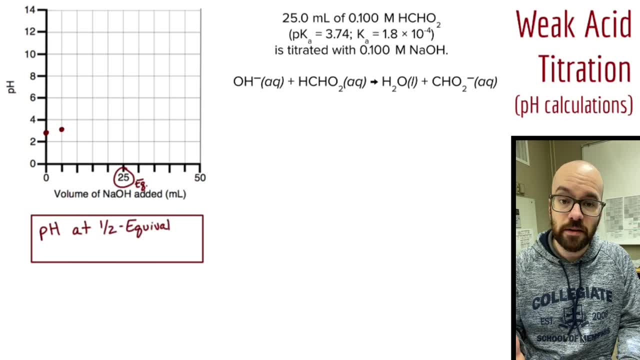 calculate the pH All right up next. now let's add some more base till we hit the half equivalence point. How do we know when we hit the half equivalence point? Well, the equivalence point was 25 milliliters of base added. The half equivalence point is half of that, So 12.5. 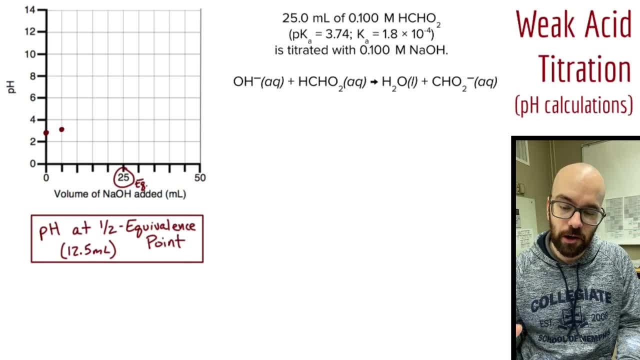 milliliters. This turns out to be the easiest one in this whole titration curve, And that's because at the equivalence point the pH is always going to be equal to the pKa. That's always going to be true for a weak acid in a titration curve. So in this case our pKa is 3.74.. So that's our pH at. 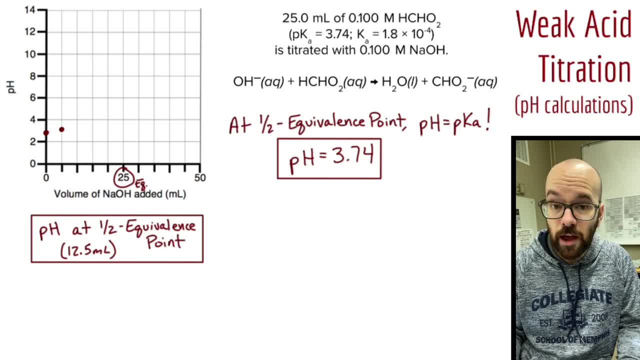 the half equivalence point. Now why is that? We can actually show that in the Henderson-Hasselbalch equation. Here we have pH equals pKa Plus log of base over acid. Now think about it. If we're at the half equivalence point, 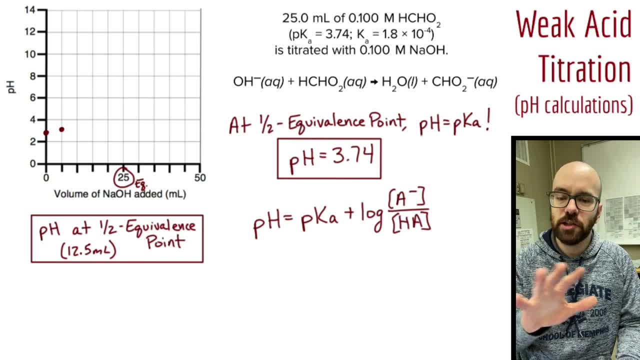 we've titrated half of the acid. So let's say just real easy numbers, real quick. Let's say we had 10 moles of the acid and we titrate half of it, Well, how much acid would we have left? 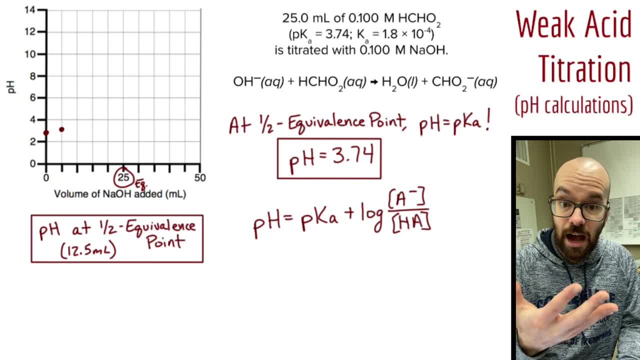 Well, we started with 10. We titrated half of it. We've got five moles of the acid left. Okay, well, what about the base? Well, that five moles of acid got converted into five moles of base. So the moles of acid and the moles of conjugate base are equal to each other. 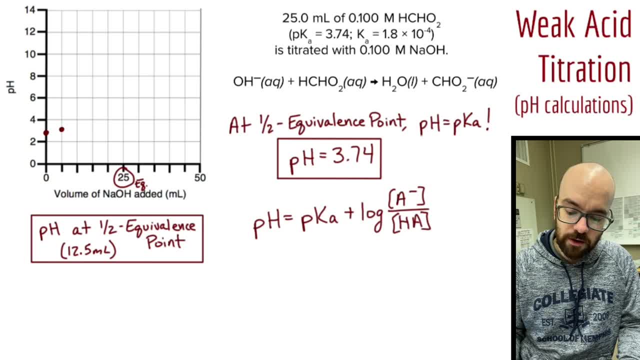 At the half equivalence point. Great. So what does that mean? for a Henderson-Hasselbalch equation That means that this, the conjugate base, equals the conjugate acid concentration. So this and this are the same. This would be log of one, and log of one is zero. So pH equals pKa. This is especially. 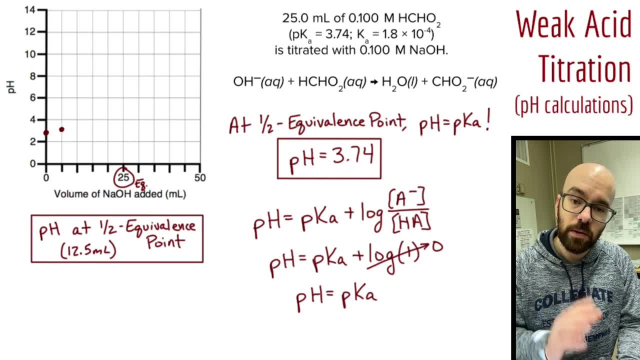 important to remember. It's a special point about a weak acid titration curve. pH equals pKa at the half equivalence point. Write it down, get it tattooed on your hand somewhere. You won't regret it. I mean, maybe you will. 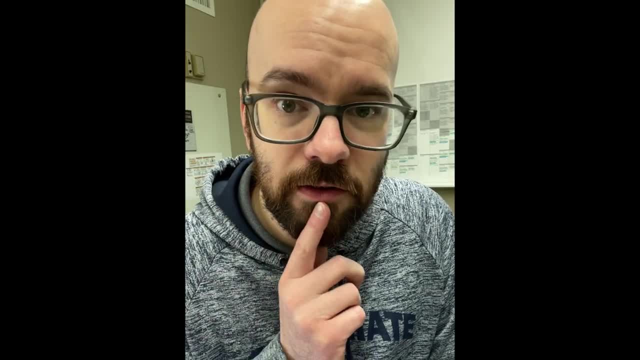 Disclaimer: if you're one of my students, don't go get that tattoo. I don't want to have to explain to a parent why. All right, let's plot that point on our titration curve- 12.5 milliliters, right. 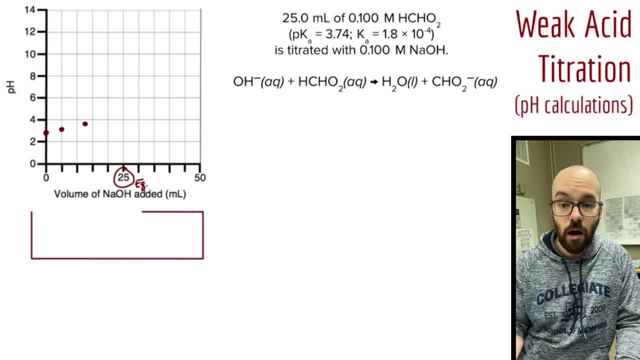 there, And that's a pH of 3.74.. All right up. next, let's add a little bit more. In this case, we've added 20 milliliters. We're still before the equivalence point, So we'll do it just like we did. 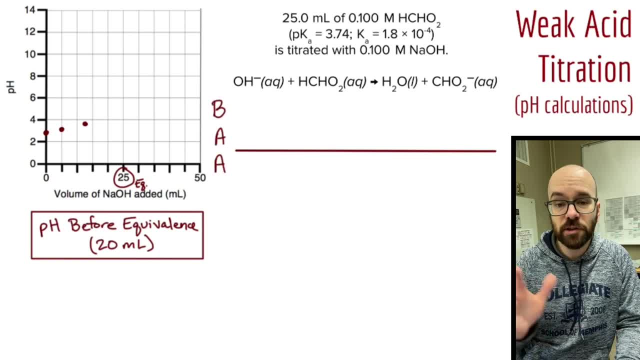 the five milliliters one. We're still before the equivalence point, So we'll still set it up exactly the same. I've got my before and after table to do my stoic calculation: Zero of the 0.0025 moles of the formic acid and approximately zero of the conjugate base to start, And then we're. 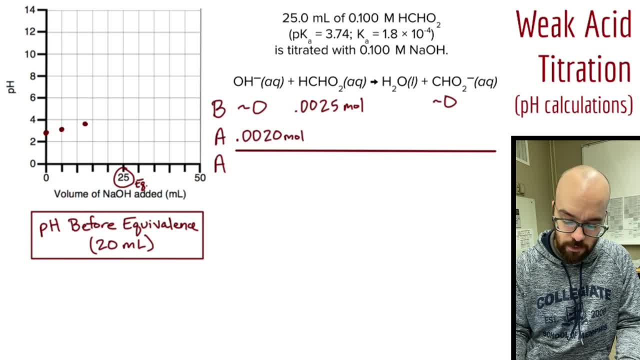 going to add 0.0020 moles of the hydroxide And of course we'll have 0.0005 moles left over of the acid. We've got 0.0020 moles left over of the conjugate base And at this point we just 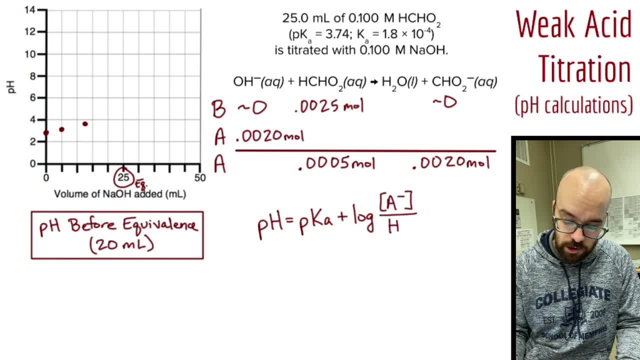 substituted in to the Henderson-Hasselbalch equation. So I'll rewrite that equation out right here, And then I'm going to substitute those two values into my equation. So my base was 0.0020.. And my acid was 0.0005.. And then I'll just put that into the calculator. I got a pH of 4.34.. 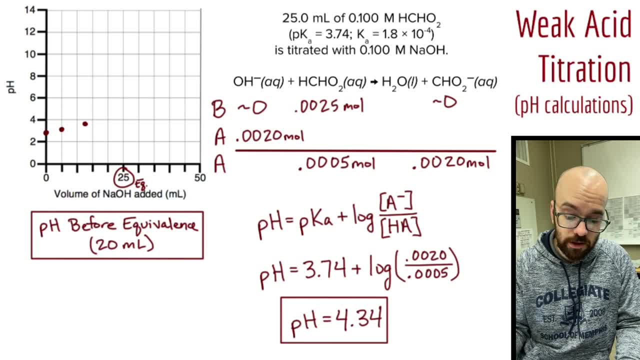 That pH is still increasing. It's not increasing a whole lot, but it is increasing, which makes sense because we're adding base. I'll plot that on my titration curve right here And so we've got kind of a nice straight line. It's a little bit steeper than the strong acid, strong base titration. 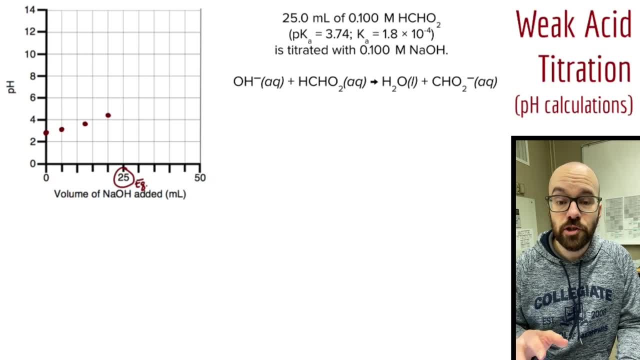 curve was. So if you've noticed that, that is a difference here. Now let's jump to the equivalence point. If you remember from strong acid, strong base titrations, the equivalence point is the easiest pH to calculate. It's always 7, but not here. That's only true for strong. 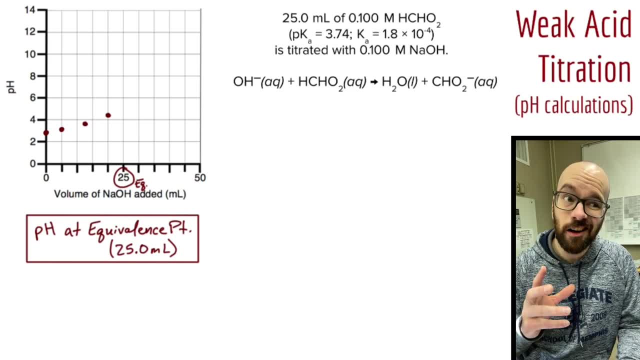 acid. strong base titrations For the weak acid. it's actually the hardest calculation. It's the most involved. So buckle up. Here we go. Equivalence point of weak acid. Here's how you do it. So let's start with a before, add after table and just see what we get. 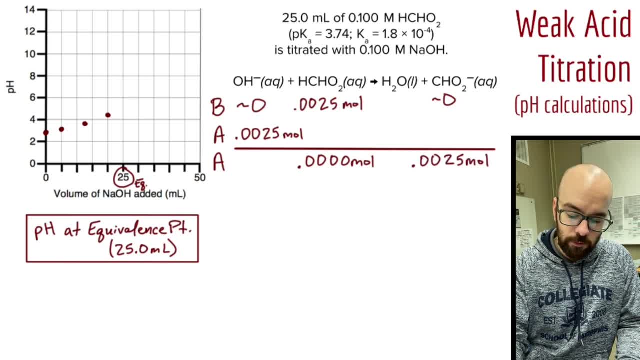 So we're at the equivalence point. It's going to look like this. I filled that in really quickly. Let's take a look. I've got 0.0025 moles of the acid, but I've reached the equivalence point. 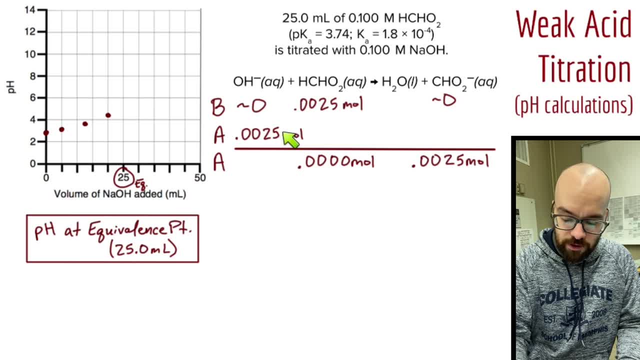 I've got an equal number of moles of hydroxide, So all of this gets neutralized. I have zero left over of my acid. It's all been converted into conjugate base. Now if I had passed the equivalence point, I would have some excess hydroxide, which would be great I could calculate. 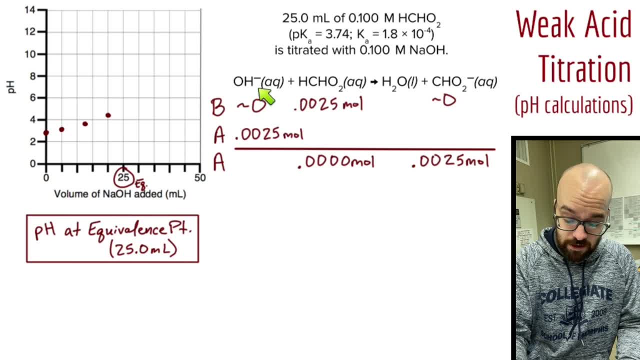 pOH, and then we're good. But I don't have any leftover hydroxide concentration. All of the hydroxide added is neutralized by the acid. I'm left with zero here. Now, your first thought might be: well, let's just substitute this into the Henderson-Hasselbalch The problem. 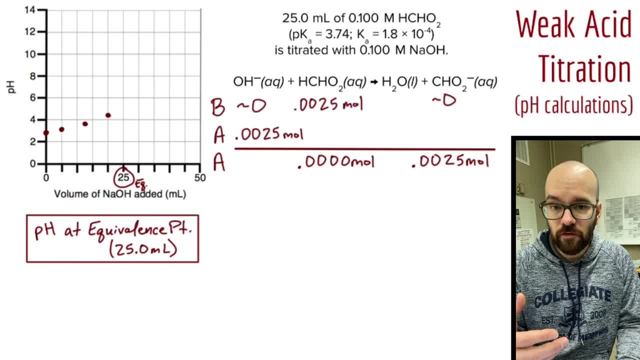 is, If either of these numbers is zero, we get an undefined log value, and that's not going to be helpful to us. You also might be tempted to think: well, we don't have any of this acid left. There's no OH. Well, aren't we just at pH seven? The problem with that is we've created this formate. 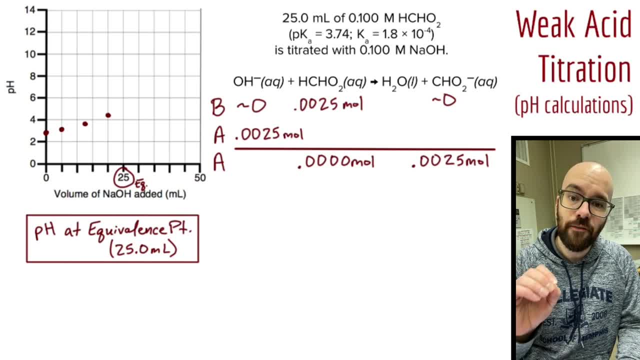 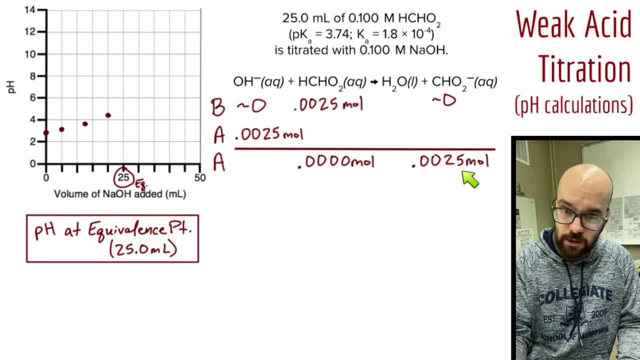 So what we need to do is think about what does this left-over formate do in water? How does it react? So first let's calculate what that formate concentration is. We just have the moles of formate right now, so the concentration of formate is going to be the 0.0025 moles divided. 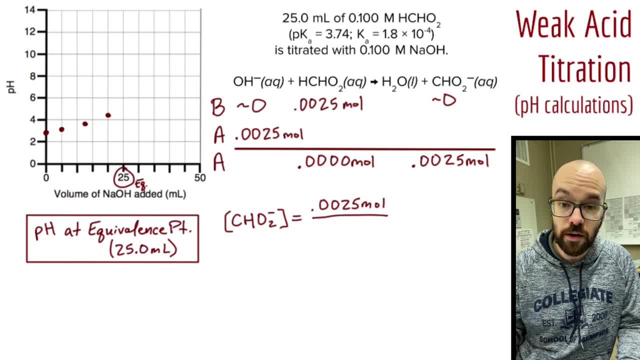 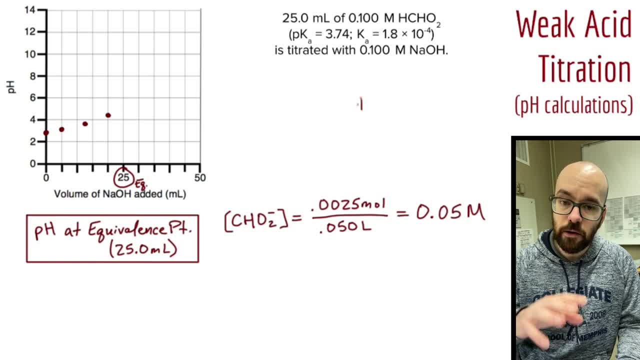 figure out. what does the formate do in water? So I'm going to rewrite out a new equation, this case with formate plus water, and what's going to happen here? Well, the formate, of course, can accept a hydrogen from the water, So it's actually going to produce some of the formic acid. 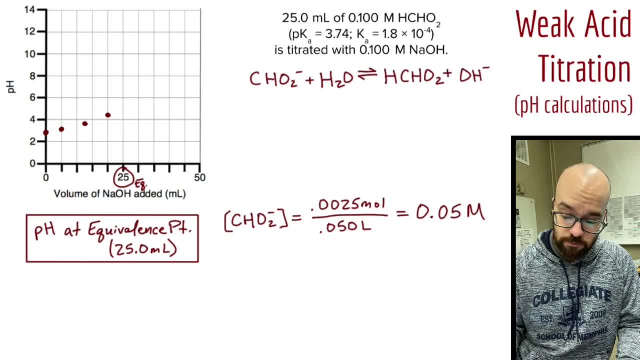 back and we'll have you left over with hydroxide. Now you might see where we're going with this. We're going to set up an ice table for this reaction and figure out what that hydroxide concentration is going to be. The hard part is kind of over there. The hard part was knowing to. 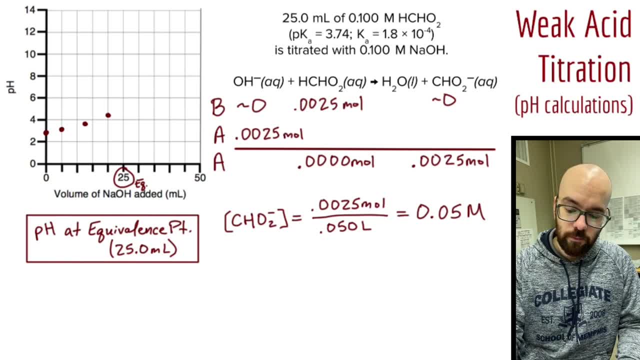 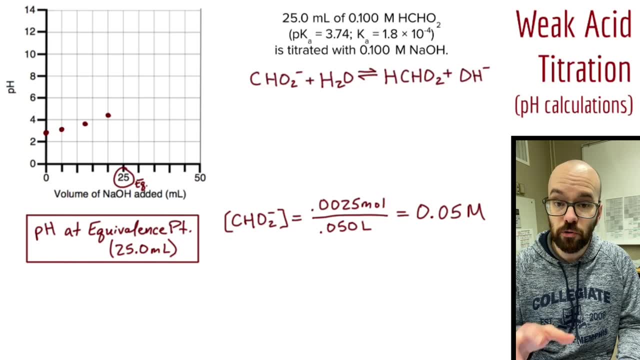 set this equation up, But remember, we got this by creating this. before and after table We saw that we had moles of formate left over and now we're just figuring out: okay, what does the formate do in the water? Then we write this reaction out and then we'll do our ice table. 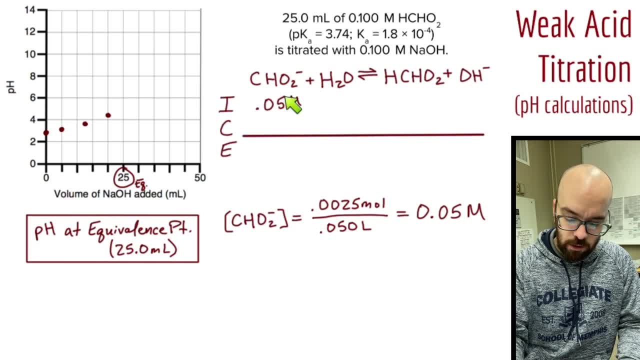 So we'll set up the ice table. It looks like we've got 0.05 molar of the formate- We got that from this right here- and then zero of both of the other ones. It's just a normal ice table situation here. And of course we've got 0.05 molar of the formate. So we've got 0.05 molar of the formate And of course we've got 0.05 molar of the formate And of course we've got 0.05 molar of the formate. And 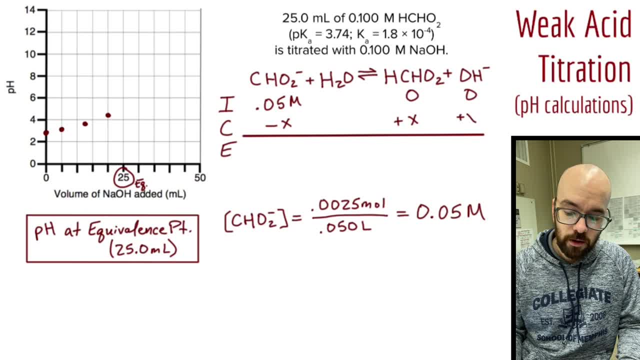 of course, the formate is going to decrease by some amount. we'll call x, The others will increase by x, and we've got our equilibrium values right there. Now this is not an acid dissociation, It's a base dissociation. So we can't use Ka for it, We've got to use Kb. Luckily, we can convert from. 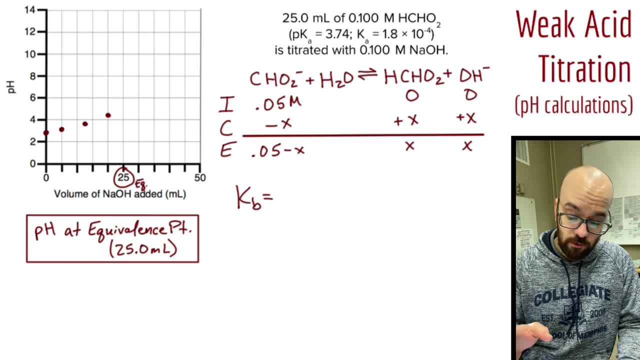 Ka to Kb pretty easily. Our Kb expression, of course, is x squared over 0.5 minus x, And let's say that the product we changed is not an acid dissociation. We've got x squared over 0.5 minus x. 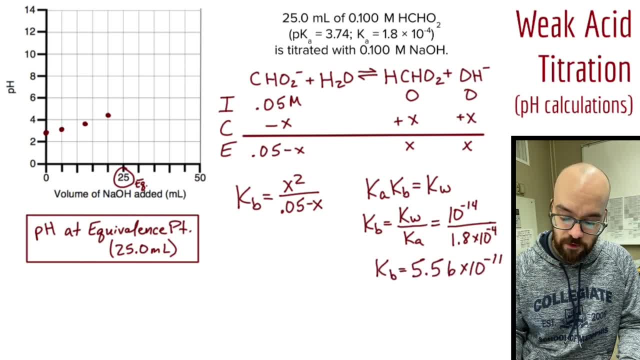 I'll substitute that into the calculator and I get a Kb equal to 5.56 times 10 to the negative 11th. There's our Kb. I can use that to calculate x, and then we'll have our hydroxide concentration. 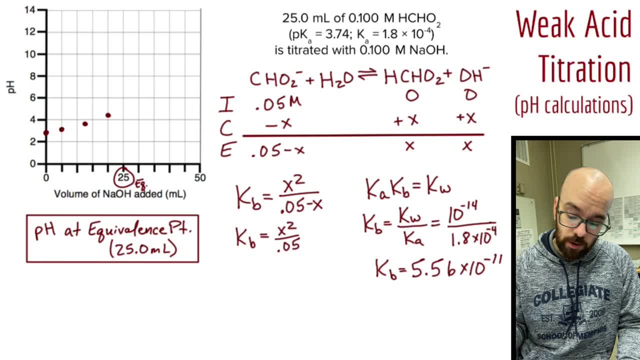 and then we'll be good to go from there. So I'm going to rewrite this with the change is small approximation. We do have a very small Kb, so this approximation is valid And then we'll just solve for our x. there, x equals the square root of 0.05 times the Kb. 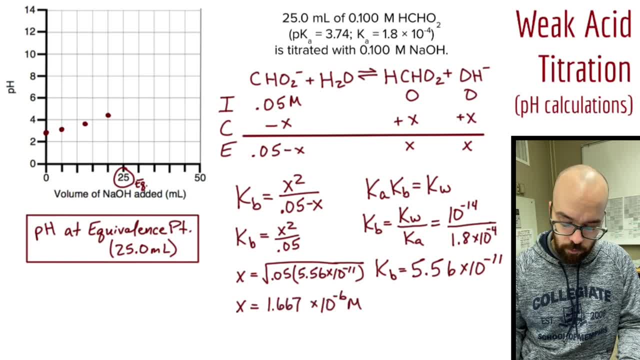 Enter that into the calculator and we'll get. x equals 1.667 times 10 to the negative 6th molar And that is our hydroxide concentration. We can take negative log of that to get pOH and that is going to give us 5.778.. 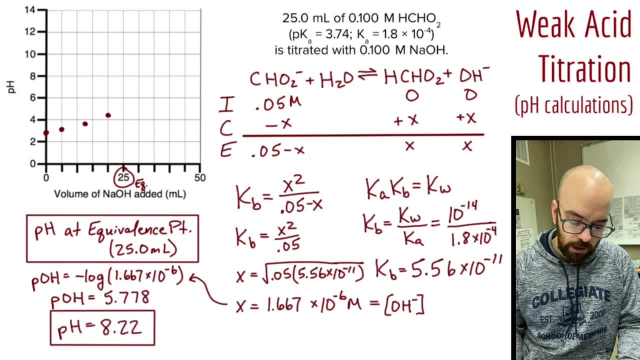 Take 14 minus the pOH to get the pH and we're going to get a pH of 8.22.. Finally, at the end of all of that, 8.22 is our pH at the equivalence point. So I'm going to. 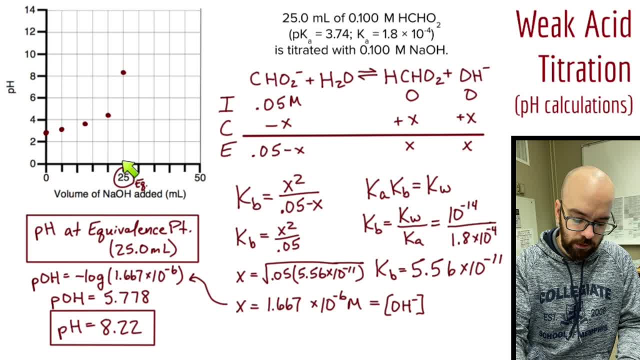 Plot that point. It goes right here at our 25 milliliters. and there's our equivalence point, pH. Again, how did we get there? We started with the before-add-after table. There's our stoichiometry calculation. It's all that. we had only the formate left. 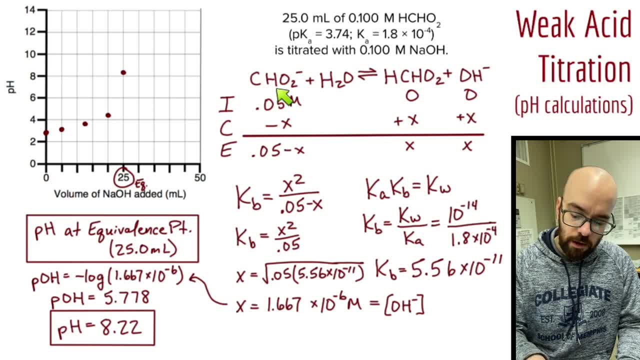 We calculated the concentration of the formate. Then we wrote out a reaction of formate in water. We added the concentration right there. We solved our ICE table to get this And of course we had to calculate Kb from our Ka using this equation. 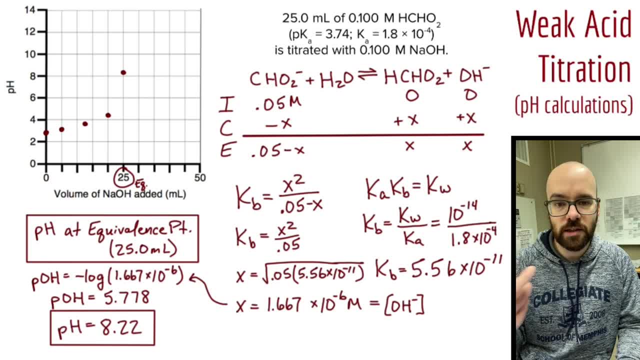 And that gave us our hydroxide concentration. Then we just did our normal pH calculations to find the pH from there. Okay, that was a lot. Let's go to another calculation after the equivalence point, But hopefully this one will feel a little bit familiar if you've done strong acid-strong base titrations. 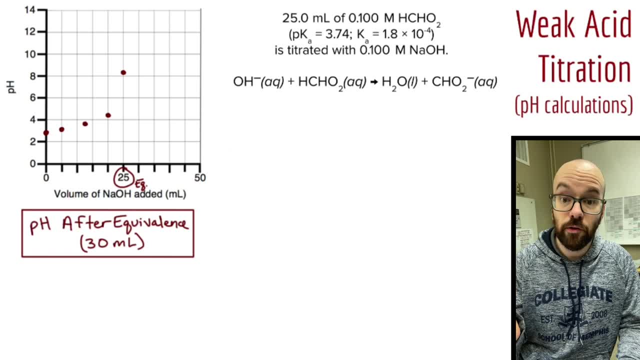 because it actually ends up being the same thing after the equivalence point as it was for the strong acid-strong base. In this case, we've added 30 milliliters. We're clearly past the equivalence point of 25 milliliters, And so we'll just start off with our before-add-after table. 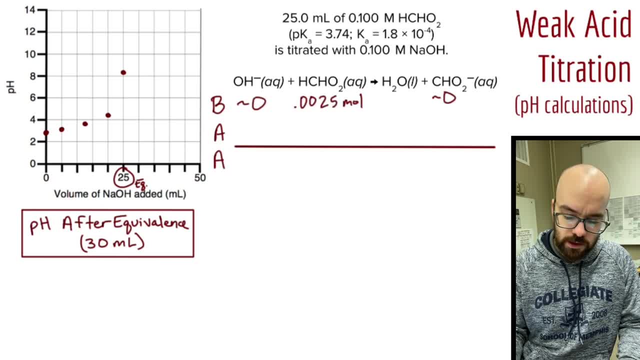 like we've done a million times at this point. So we've got this. to start off, with our 0.0025 moles of our acid, We added 0.0030 moles of our base. Of course. we got that by taking 30 milliliters. convert to 0.030 liters. 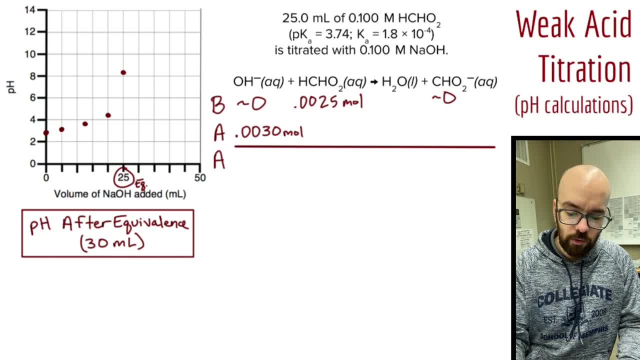 multiply that by the concentration of our base. All right, so what do we have left? Well, all of this gets neutralized. We'll be left with 0.0005 of the hydroxide, zero of that, And we've got 0.0025 moles of the formate. 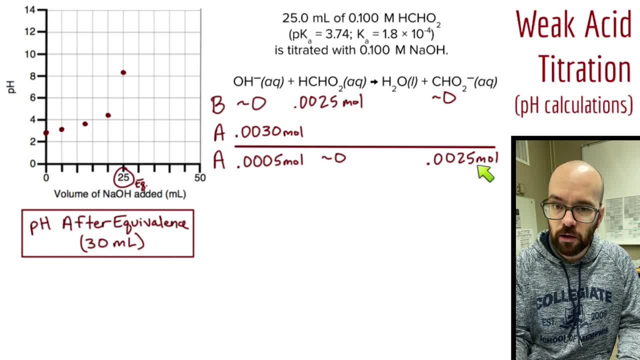 But here's the thing: The formate has relatively little effect compared to the hydroxide concentration. So if we get a hydroxide concentration number, we can just use that to calculate the pOH and then the pH. So we're not worried about this, like we were in the equivalence point. 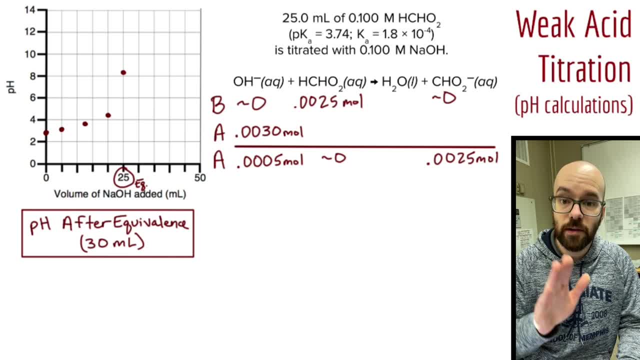 Because we have this excess hydroxide, we can just use that to calculate the pOH and the pH. So we've got 0.0005 moles of hydroxide. We'll calculate the hydroxide concentration 0.0005 moles. 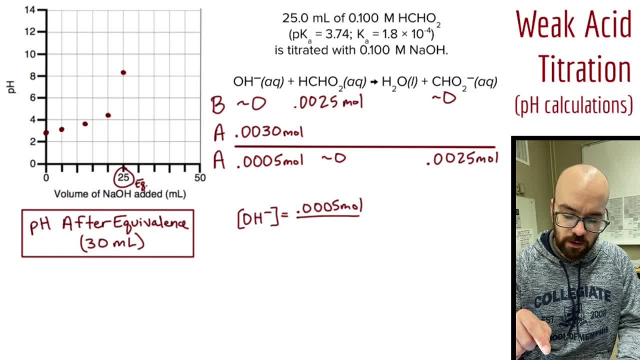 We'll divide by the volume. We had 25 milliliters and we added 30,, so that's 55 milliliters. So divide by 0.055 liters We get 0.0090 repeating molar for our hydroxide. 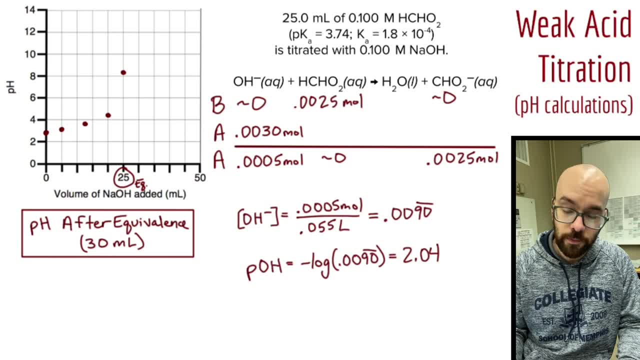 Take negative log of that, We get a pH of 2.04.. 14 minus that, we get a pH of 11.96.. I'll graph that on my titration curve at 30 milliliters, up here just under 12.. 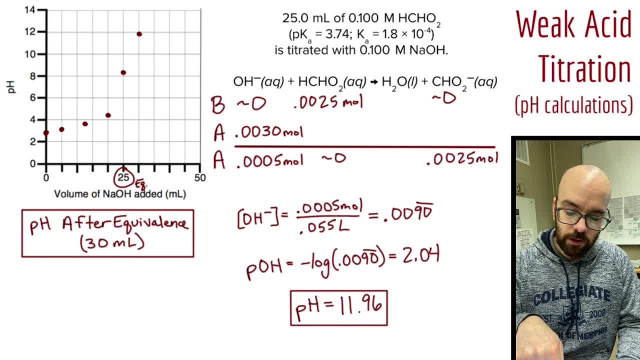 For sake of time, I'm not going to calculate the next point. Okay, I'm going to do 40 milliliters. If I calculated it, though, I would just follow all of this procedure again for the different volume. At 40 milliliters, we get a pH of 12.3 something. 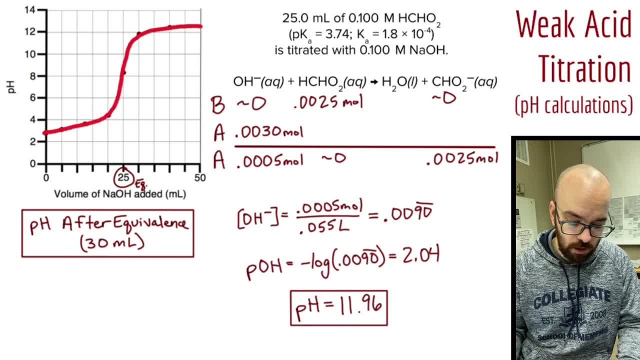 It's right in there. We've got our nice S-shaped titration curve right there. Now there's two important points that I want to just go ahead and mark on the titration curve that we have. The first, of course, is the equivalence point. 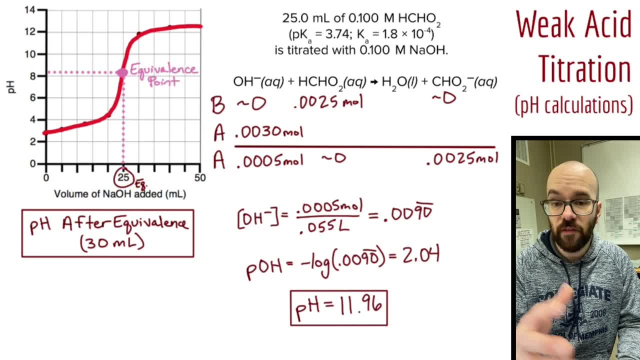 We know the equivalence point has a volume of 25 milliliters. In this case we found that with MV equals MV at the very beginning And we know that equivalence point pH value is going to be 8.22.. If I just had the graph and no calculations or other data. 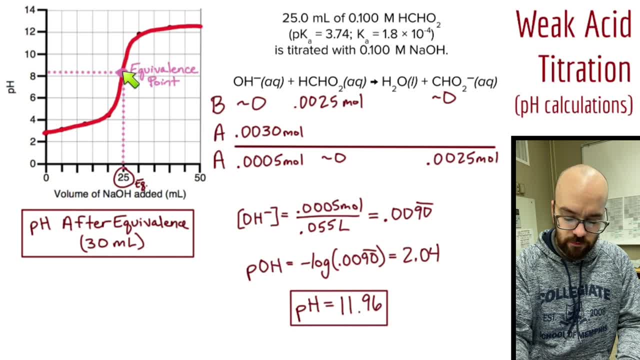 I could find where this point is right here, where it's kind of the most vertical, and go over here to estimate what that equivalence point, pH, would be. The second point, just as important, for us, is going to be that half equivalence point. 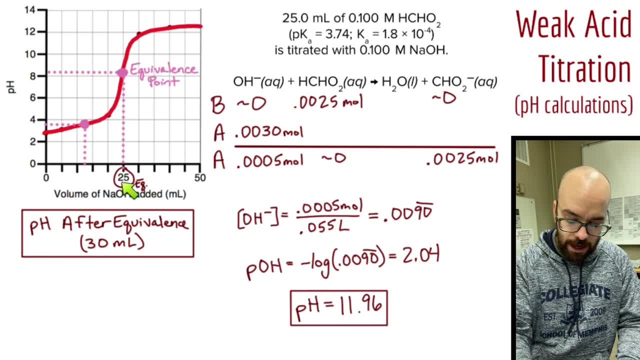 To get the half equivalence point volume, just divide the equivalence point volume by half. That's going to be 12.5.. And of course I can find the pKa for my graph if I find this point and I just follow it over on the graph right there. 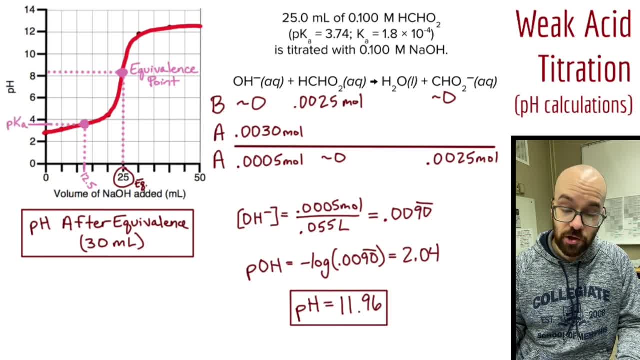 That's going to give me my pKa, And that's going to give me my pKa, And that's going to give me my pKa, And that's going to give me my pKa. In this case, of course, was 3.74.. 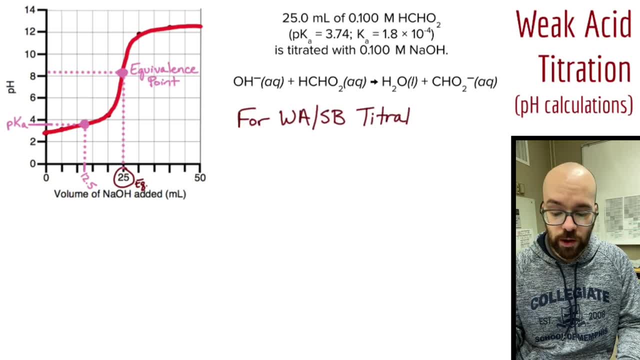 So remember that half equivalence point- very important. Now let's do a quick summary for weak acid strong base titrations. How did we get the initial pH in this titration curve? Well, we did an ICE table because we just had a weak acid that we started with. 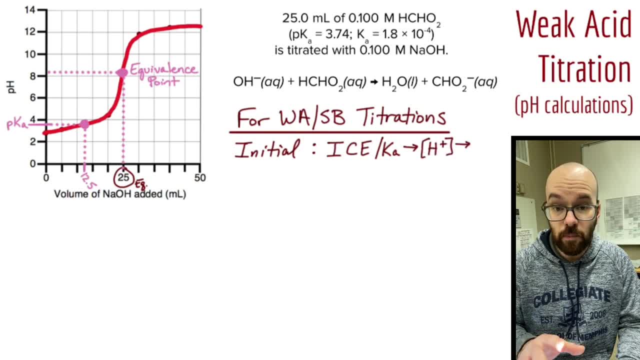 We did an ICE table, our Ka expression. We calculated the H plus concentration from that and then to the pH. OK, what about when we're before the equivalence point? We've added some base, but we're not to the equivalence point yet. 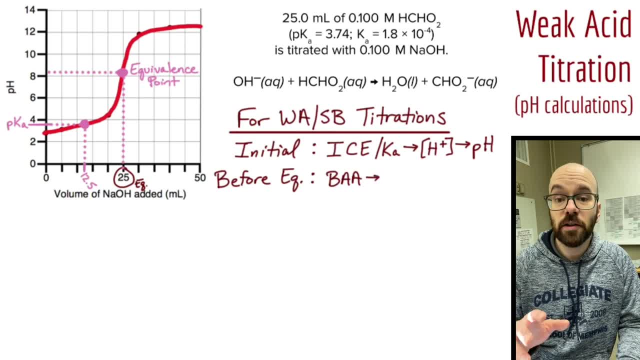 First thing that we always start off with is going to be our before add after table. That's going to give us the concentration of acid left over, as well as the conjugate base. We can use that data in the Henderson-Hasselbalch equation. 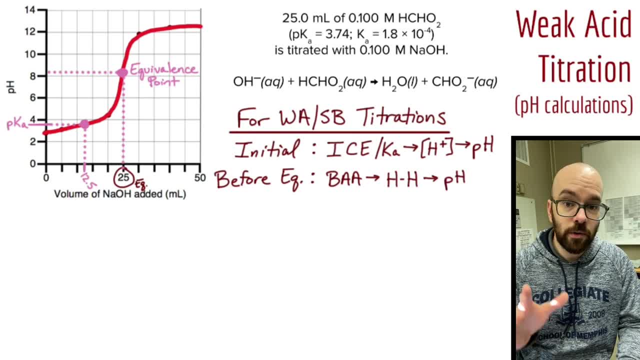 which gives us the pH. Now there's a special case. remember, at the half equivalence point. How do we find the pH at the half equivalence point? Well, we remember that the pH at the half equivalence point is equal to the pKa. 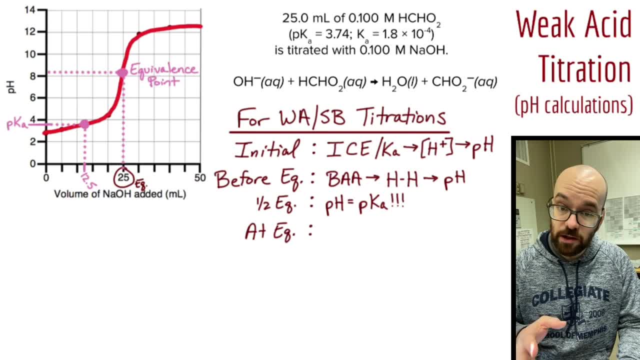 Simple as that. But remember that It's really important. How do we find the pH at the equivalence point of a weak acid titration? This is the big one that takes a long time. It takes a long time, But how we do it is we take the conjugate base. 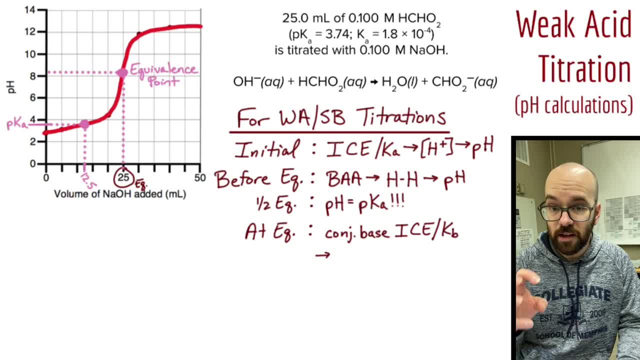 We do the ICE table based on the conjugate base And we use the Kb. We use that to calculate our hydroxide concentration. This requires us writing a reaction of conjugate base plus water. It gives us some products. We do the ICE table, Kb, all of that.